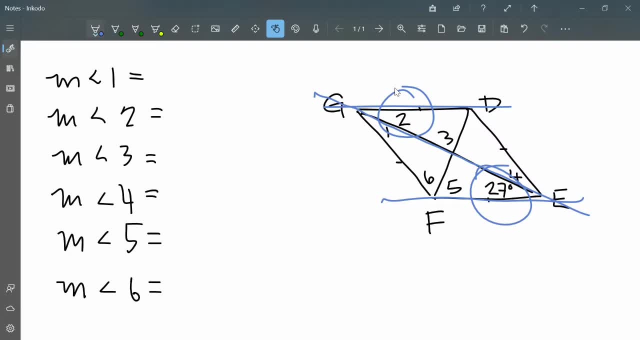 which have the same measure. So the measure of angle 2 is 27 degrees. Let me remove my markings there. It is also a fact that diagonals bisect the angles in the rhombus. So the measure of angle 1 is the same as the measure of angle 2, which is 27 degrees. 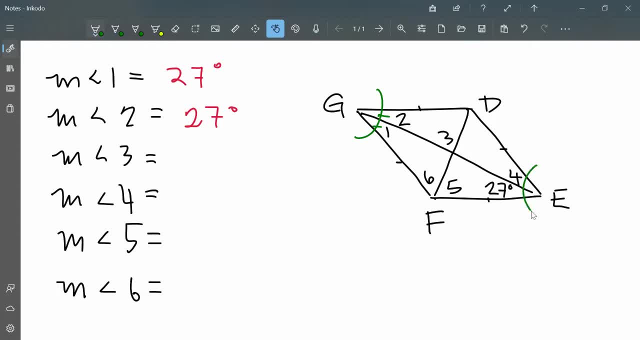 Opposite angles are congruent, so that makes the measure of angle 4 also 27 degrees. The next property we will use is the fact that in a rhombus diagonals are perpendicular, So the measure of angle 3 is 90 degrees. 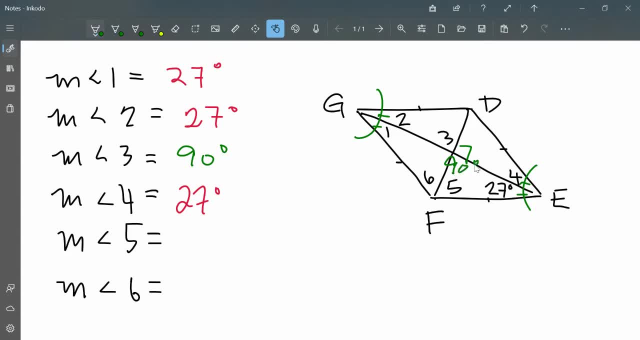 That also makes the angle in this triangle 90 degrees. So measure of angle 5 plus 90.. 90 degrees plus 27 degrees is 180 degrees. If I subtract, add angles and subtract, we find that the measure of angle 5 is 63 degrees. 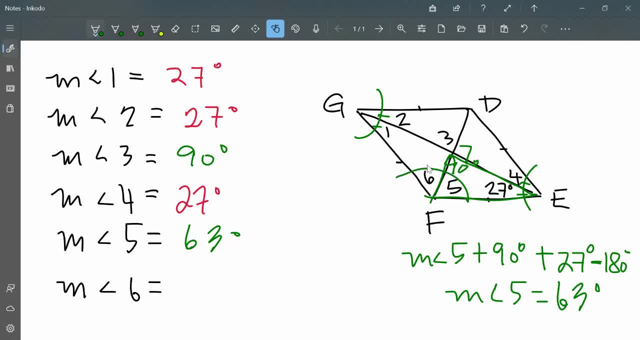 And once again the diagonal bisects this angle, making the measure of angle 6 also 63 degrees. And once again the diagonal bisects this angle, making the measure of angle 6 also 63 degrees. And once again the diagonal bisects this angle, making the measure of angle 6 also 63 degrees.